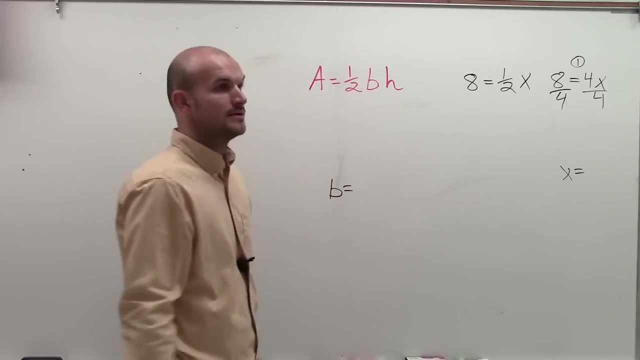 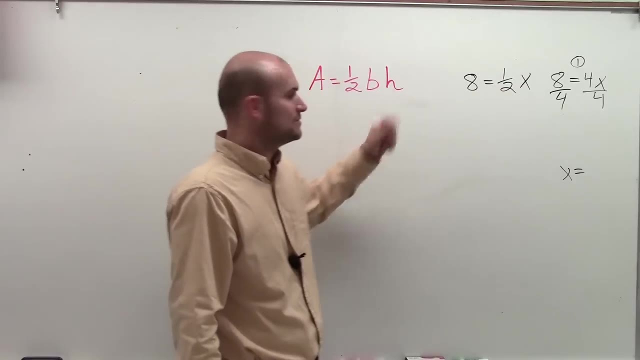 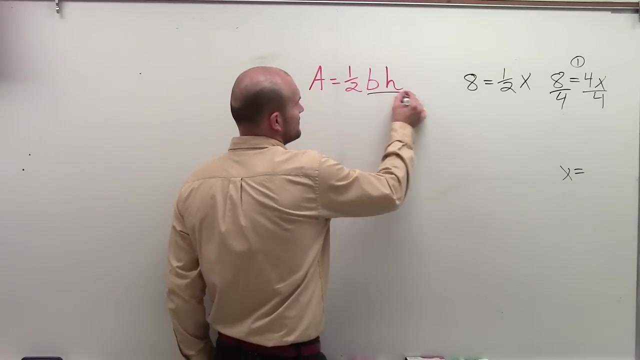 our whole goal. we're solving for b. we want to get b by itself, So we have a number that's being multiplied by b- H, right? So what do you think, kind of parallel to solving that problem, you would do with h? Right, Because h is multiplied by b. Does that make sense? Okay, So we need to divide. 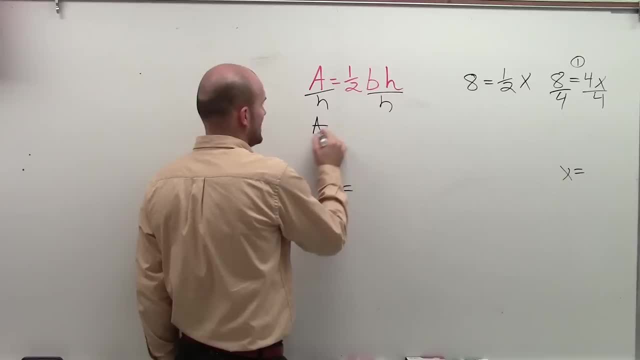 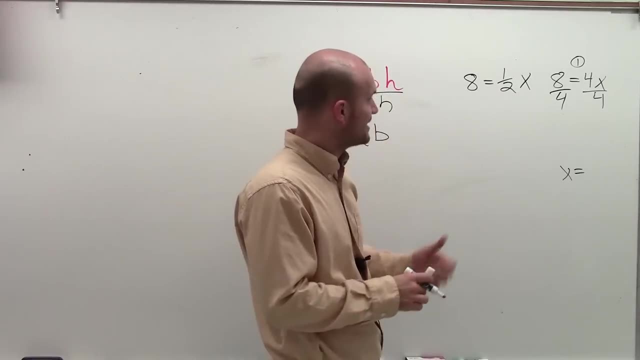 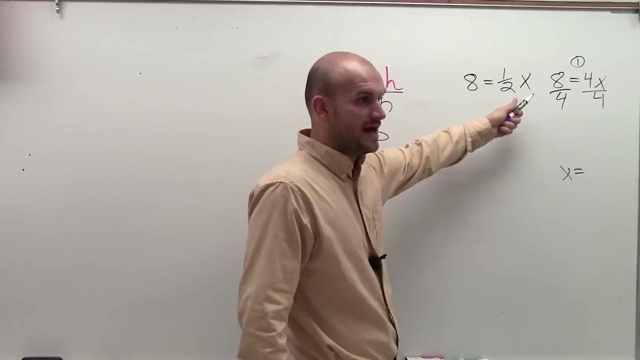 by h. So now I have a divided by h equals one half b. Now, if you remember over here, remember we were talking about how to get rid of the fraction. Now we talked about how to get rid of the fraction. especially when you have like one half x, You always want to multiply by the reciprocal. So the reciprocal. 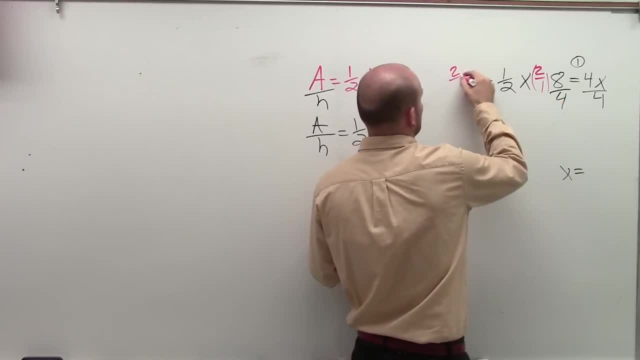 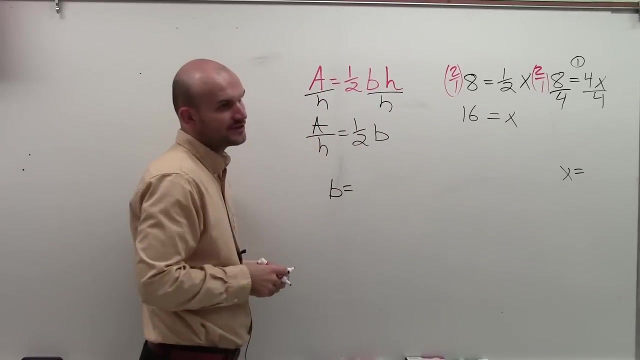 here would be two over one, So two over one. our number times its reciprocal equals. one One times x is just equal to x. One times 8 is 16.. Right, Fair enough. So here, what do you think you're going to want to do with? 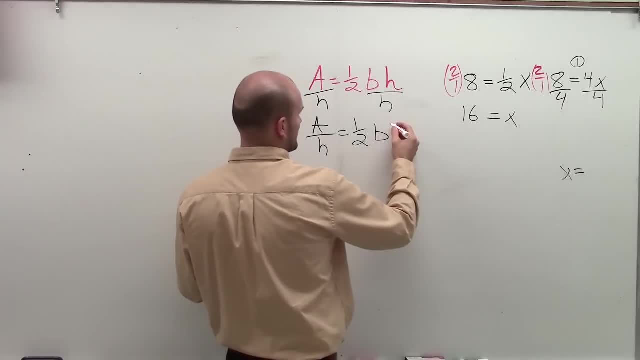 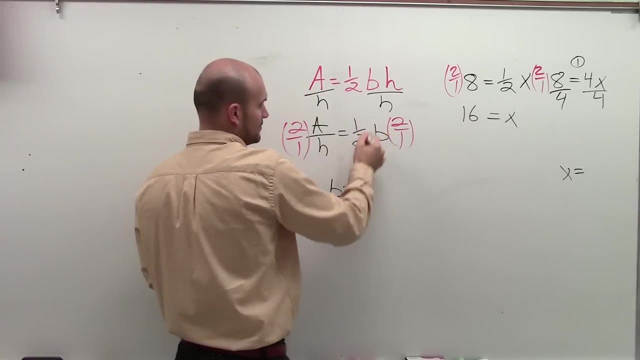 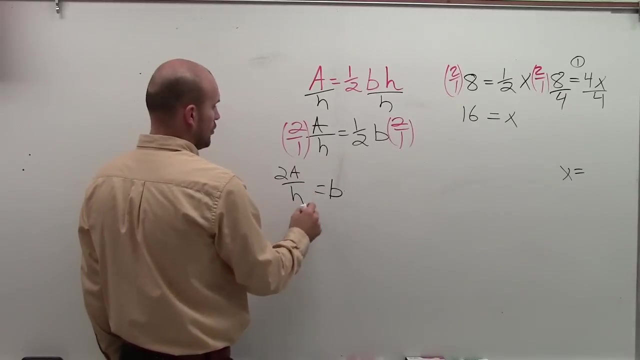 the one half b. Let's multiply by h, Or no, two over one, Right, Two over one. So therefore, again, those go to one, So you're left with b. Let's actually write it this way: b equals 2a over h, And then we always like to rewrite with our variable. 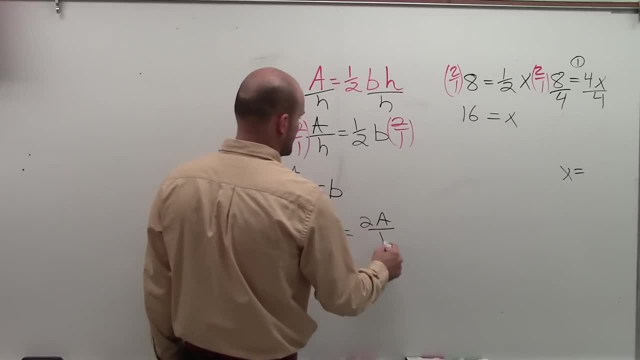 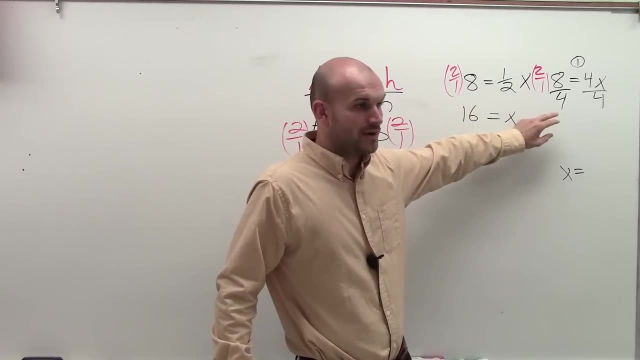 first that we're solving, for b equals 2a over h. Okay, 2a over h Make sense. So when you're doing literal equations and you're kind of getting stuck, I sometimes like to write, make up my own problems. that's going to kind of mock them, And then you just 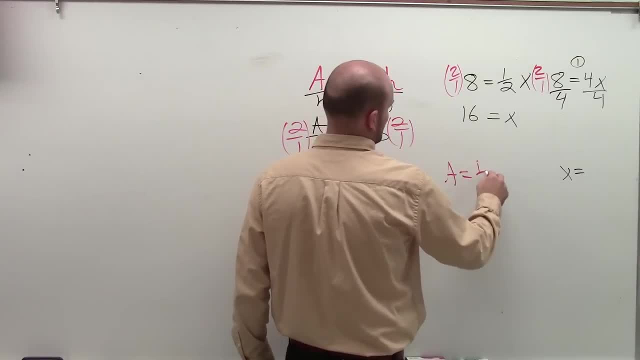 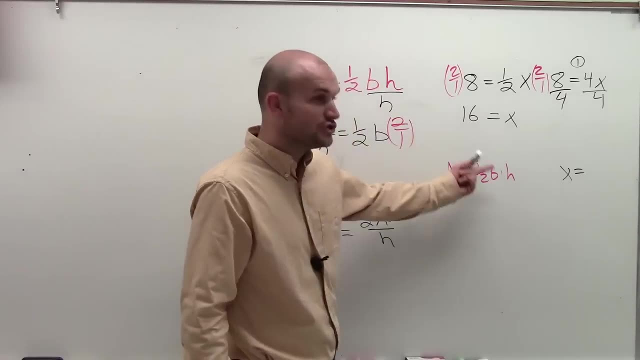 you can do them at the same time too. a equals one half b times h. Right, You don't have to. the other thing I want to tell you about is you could do these at the same time A lot of times. what other students remember is: three times four equals four times three. 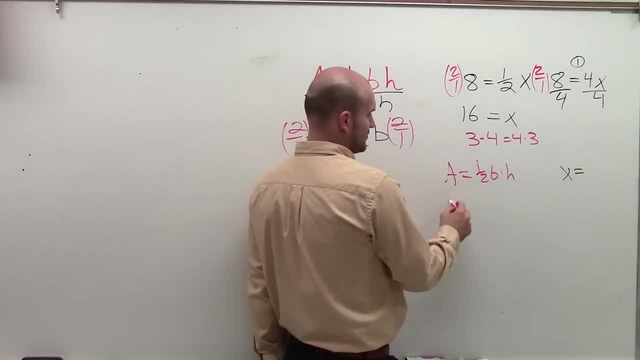 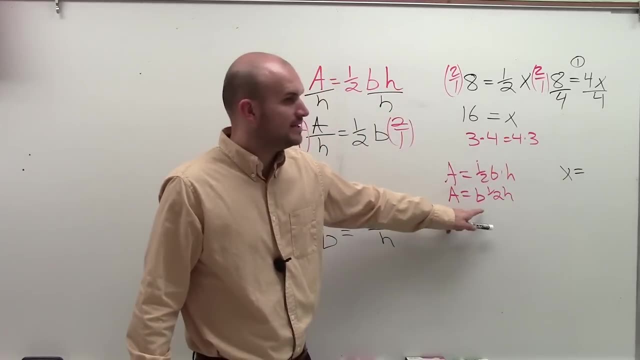 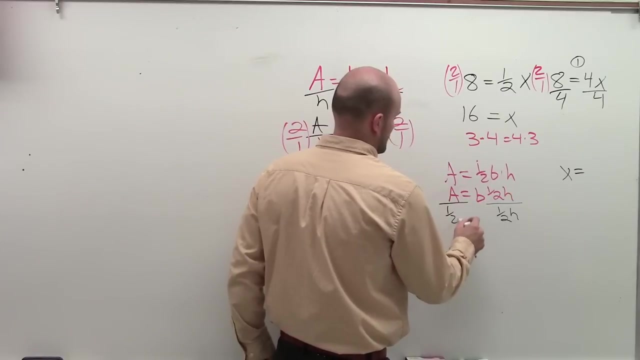 Right, It doesn't matter how you order them, So I can rewrite this as a equals b times one half h. All right, Now what is being multiplied by b? One half h. One half h? Right, So you could just do this at the same time. Well, instead of dividing.